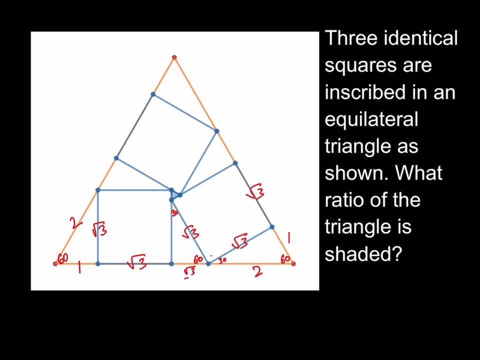 leg is half the hypotenuse, So this is going to be root 3 over 2 here, Awesome. So that basically for the equilateral. Isn't that cool, Nice, That's something that we need. Okay, So what we need to. 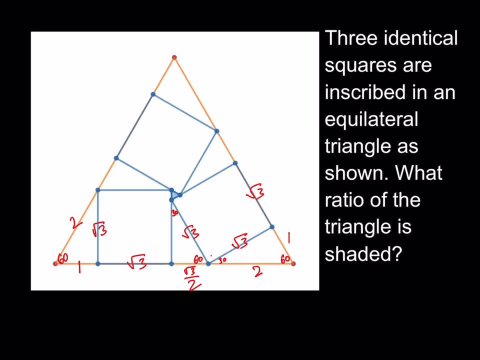 do now is find the side leg for this tiny tiny triangle here, which is the blue one. Okay, How do we find that one? Well, if the shorter leg is root 3 over 2, I multiply that by root 3 to find. 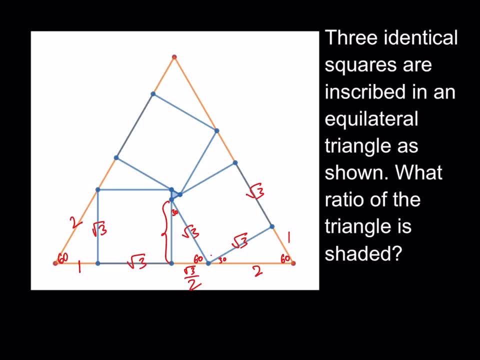 the longer leg. So the longer leg here is going to be, then what? 3 over 2.. But I also know that the whole thing is root 3 here, as you can see here, and that's a square, So all sides have the. 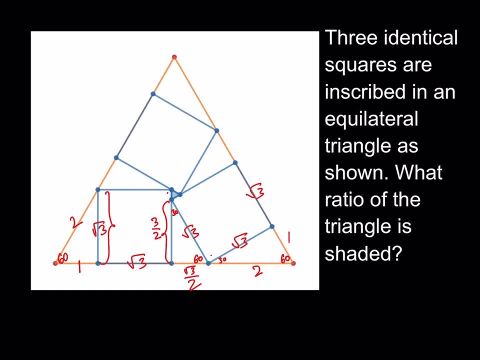 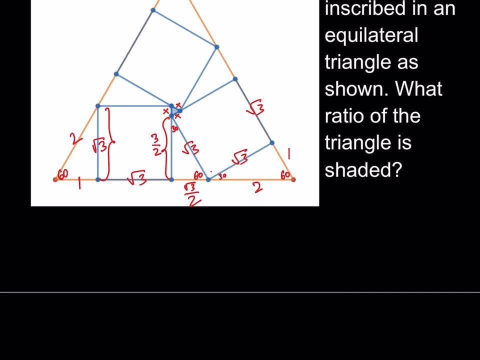 same length. Therefore, that little piece here, if you call that x, that little piece for the side length right, x, x, x, then x is going to be what x is going to be: square root of 3 minus 3 halves. 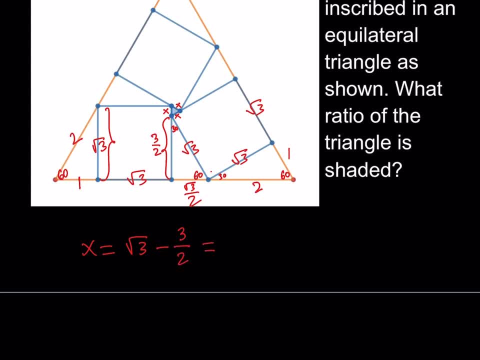 Awesome, Then what I can do is I can actually make a common denominator and write it as 2 root 3 minus 3.. So I can actually make a common denominator and write it as 2 root 3 minus 3.. 3 divided by 2.. So that would be the side length for my little tiny triangle in the middle, Okay. 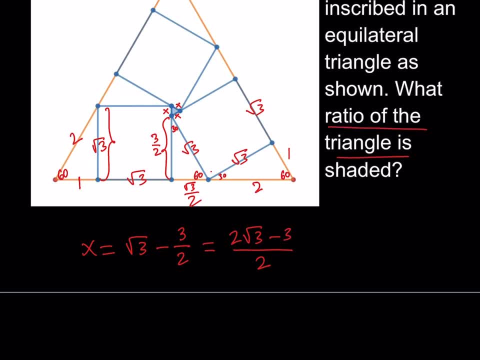 So what I need to do is I need to find the ratio of the triangle shaded. So what I need to do is find the area of the small triangle and then find the area of the large triangle and then divide them. So, but to find the areas, I do need the side lengths. and notice that for an equilateral 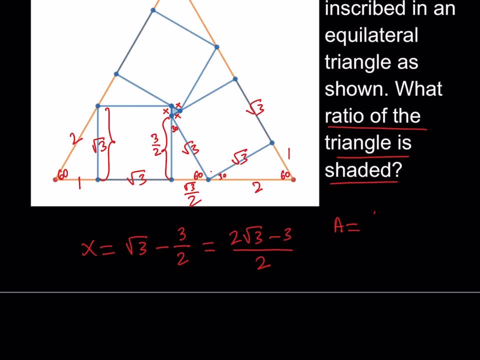 triangle. if the side length is equal to the side length, then I need to find the ratio of the side length is x, The area would be x squared multiplied by root 3 over 4.. But since both of the triangles are going to have that, we don't really care about that because they're going to 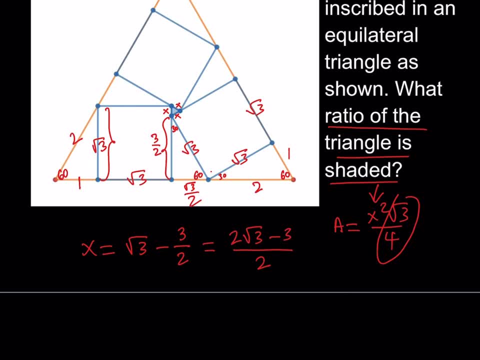 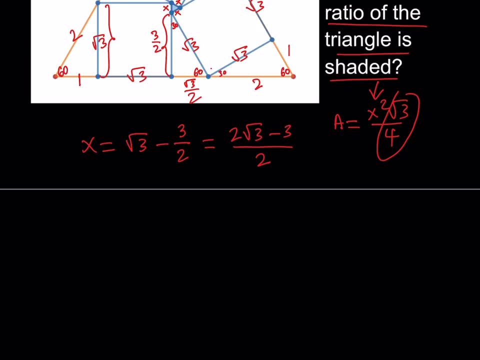 cancel out. So, basically, you're basically looking at the ratio of the side length squared. That's pretty much what it comes down to, right? Okay? So let's go ahead and write that down. The side length for the big triangle. side length for the big triangle is going to be 1 plus root 3,. 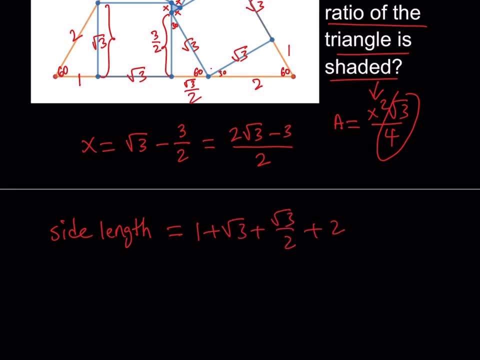 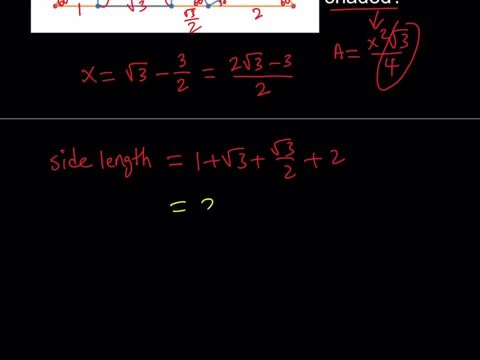 plus root, 3 over 2, plus 2.. Okay, All right. Now what are we going to do? We're going to go ahead and simplify this. Let's go ahead and simplify that 1 plus 2 can be added. That's. 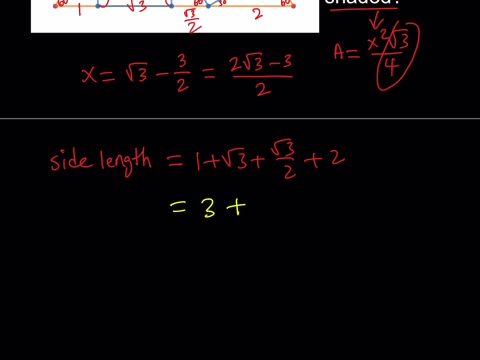 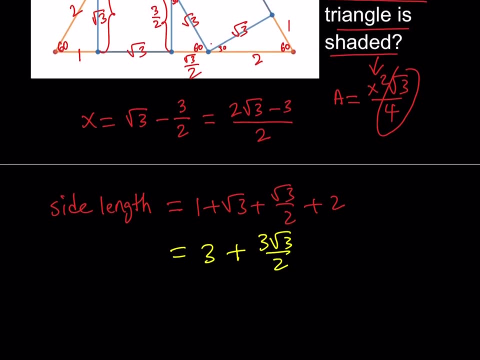 going to give us a 3.. And these two can be added as well And that's going to give us 3 root 3 over 2.. So that's my side length for the large rectangle and for the- I mean the triangle- And for the. 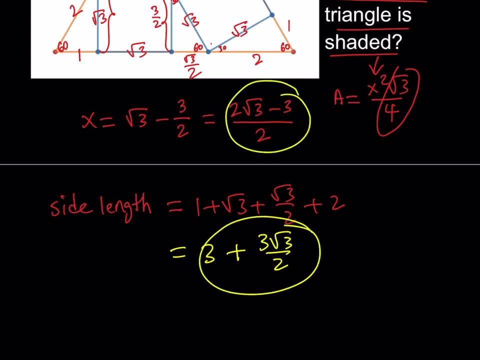 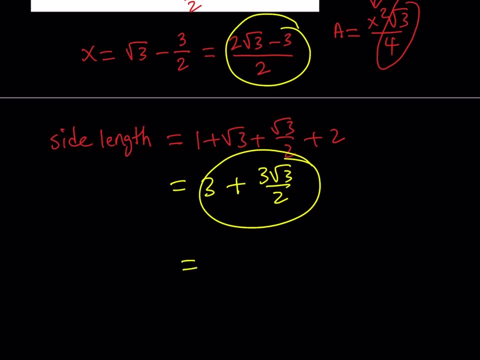 small one, it's this one. So what I need to do next is basically find the squares of these quantities, find their ratio. But before that, let's go ahead and make a common denominator here as well. So write it as 6 plus 3 root 3 divided by 2.. So that's going to be my larger length, That's going. 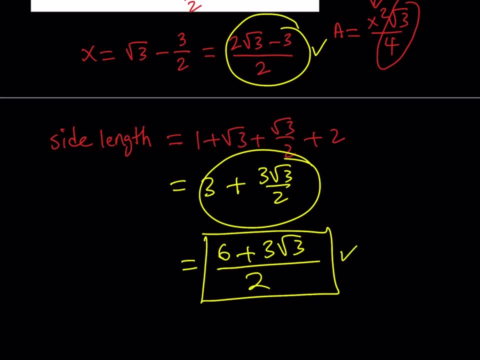 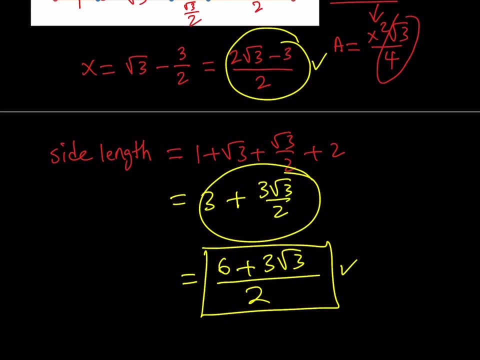 to be my smaller length And I'm going to be looking at the ratio of their squares. All right, Let's go ahead and do that. One way to do that is you can actually go ahead and find the ratio here and then square it, Or you can square and look at the ratios. Doesn't really matter, No big deal. 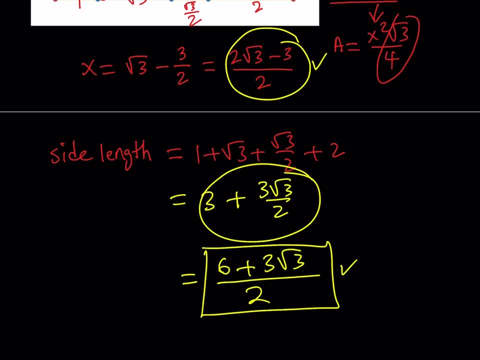 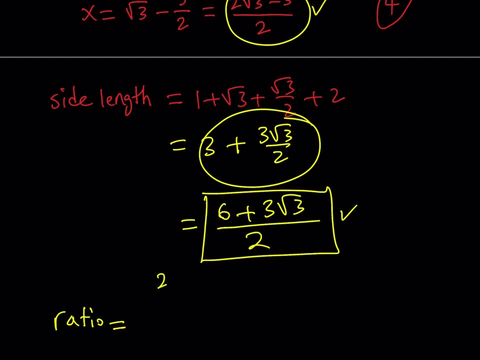 But I guess it'll be slightly easier if you just look at the ratio and then square it. Okay, So the ratio that I'm looking for is going to be then: 2 root 3 minus 3 over 2 divided by 6 plus. 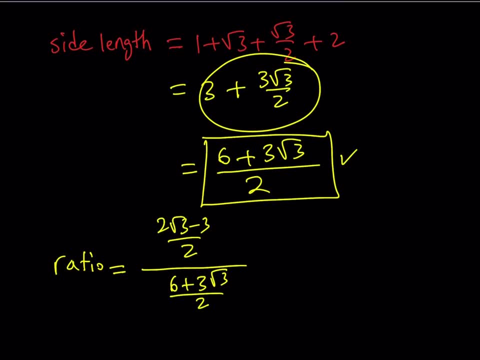 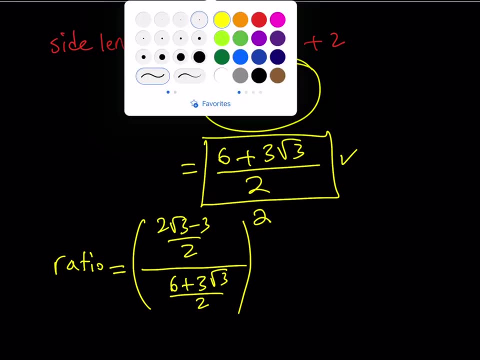 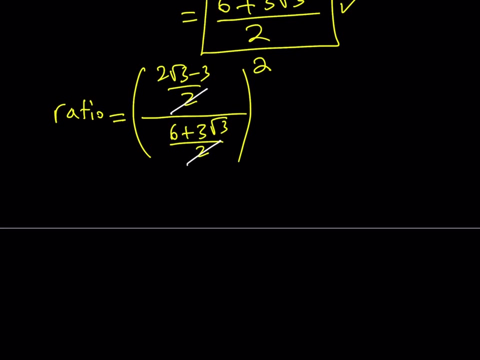 3 root 3 divided by 2. And both of them are squared. So what I'm going to do is I'm going to find the ratio first and then square the quotient. Okay, Awesome, Let's go ahead and proceed from here. The 2 cancels out. Then I end up with this. So let's go ahead and simplify that. 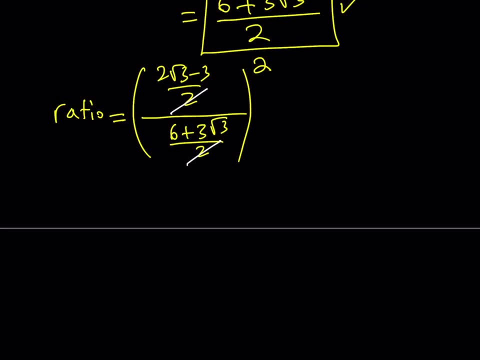 expression, And then we'll come, we'll go back and square it. So what I have is 2 root 3 minus 3, divided by 6 plus 3 root 3, which obviously can be multiplied by the conjugate. Let's go ahead and do that. 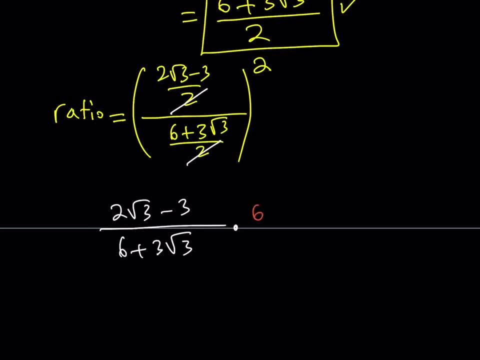 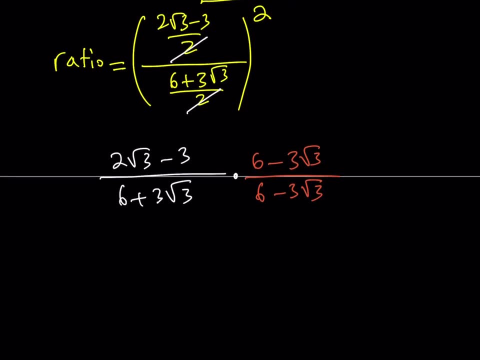 The conjugate is going to be 6 minus 3 root 3, divided by 6 minus 3 root 3.. And then the products. Let's go ahead and distribute this. This is going to be 12 root 3 minus 2 root 3 multiplied by 3. 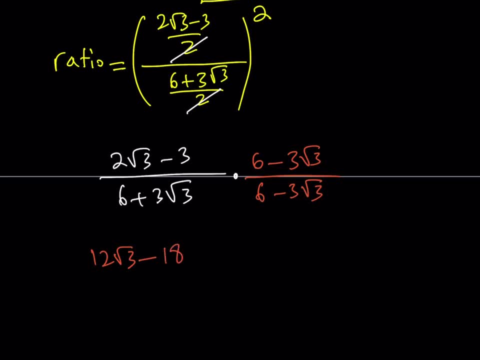 root 3 is 6 times 3, which is 18 minus 3.. And then I'm going to do that. So I'm going to do that, 3 times 6 is going to be 18 again, And then plus I'm going to get 9 root 3 from here, And then the. 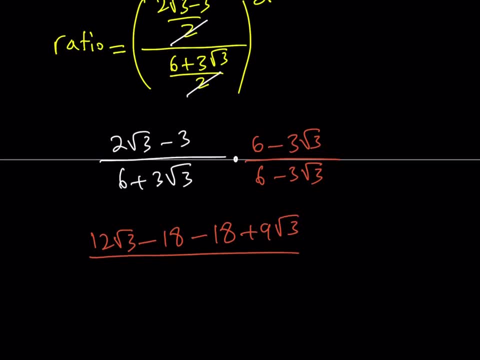 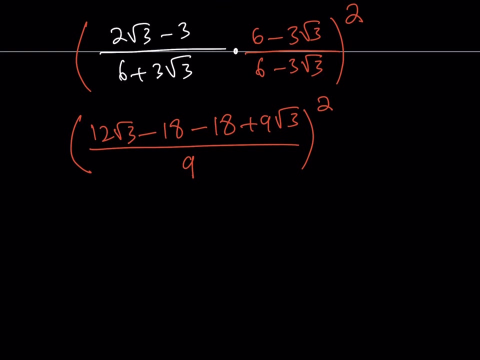 bottom is going to be difference of 2 squares 36 minus 27,, which is 9.. Awesome. Then, of course, what I need to do is I need to take that expression and square it. I need to take that expression and square it. Okay, Let's simplify this a little bit. 12 plus 9 is going to be 21. 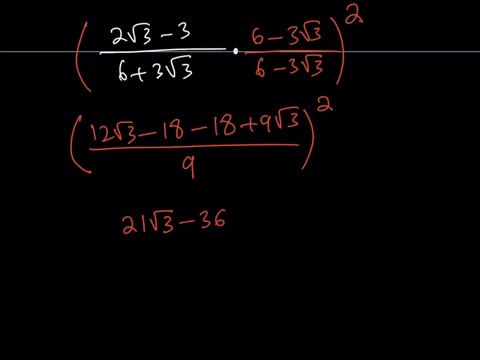 root 3 minus 36. Divided by 9, squared. Now what we need to do is- we can actually simplify this, because everything is divisible by 3.. So that'll be 7 root 3 minus 12 divided by 3.. And then we'll square that. 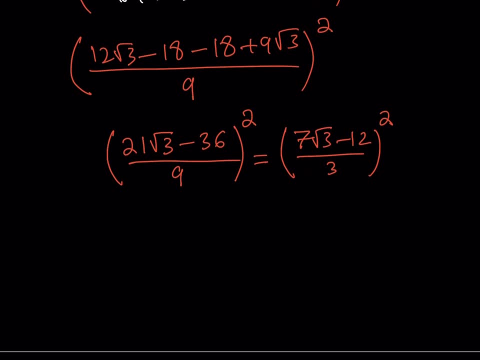 expression And then when we square the expression, it's going to look like the following: 7 root 3 squared is going to be 49 times 3, which is 147 minus their product is going to be 84 root 3,. 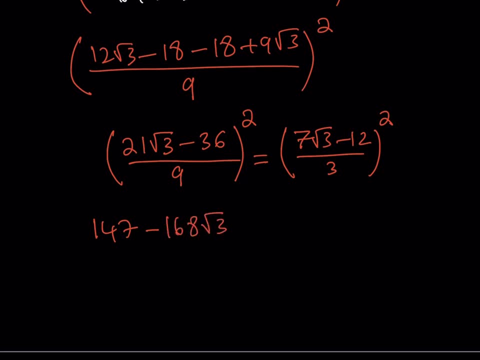 but double that: 168 root 3.. 3 plus 12 squared is going to be 144.. Okay, And then all over 9.. Obviously, what you can do is you can just go ahead and add these two quantities up. That's going to give you 291.. Okay. 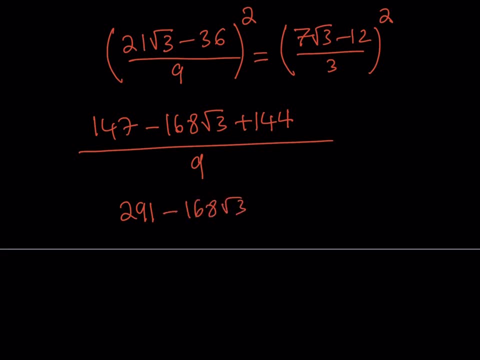 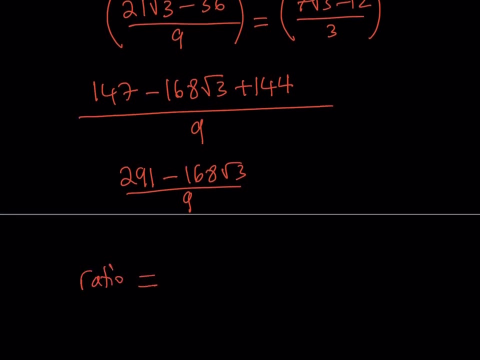 And minus 168 root 3 divided by 9.. And luckily all of these numbers are divisible by 3.. So we can go ahead and divide everything by 3 and write our ratio In actually the simplest form: Divide everything by 3.. So this should be 97.. 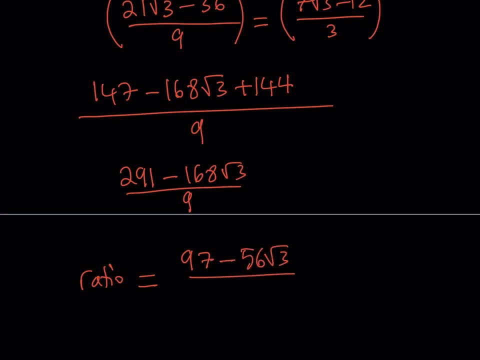 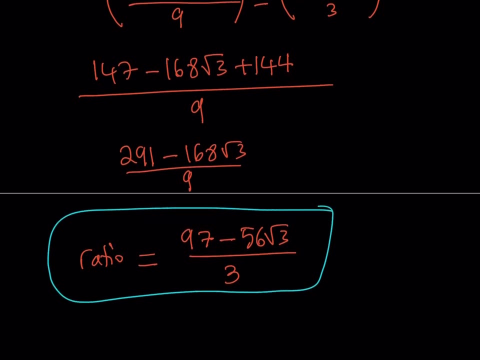 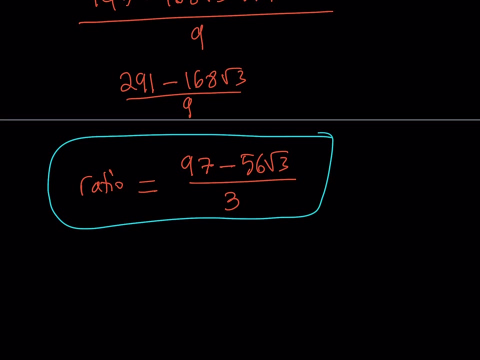 168 would be 56 root 3 divided by 3.. So, basically, this is the ratio I've been looking for And if you're wondering what that ratio is going to look like, that's actually a very, very small number And that's actually going to be something like- because, okay, it looks like a large numerator. 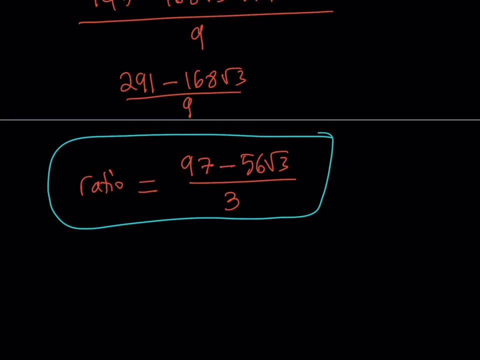 right, But the fact is that the square root of 3 is about 1.7.. When you multiply that by 56, you're going to get a number that's really close to 97.. So the difference will be very small. And if you're wondering what that's going to look, 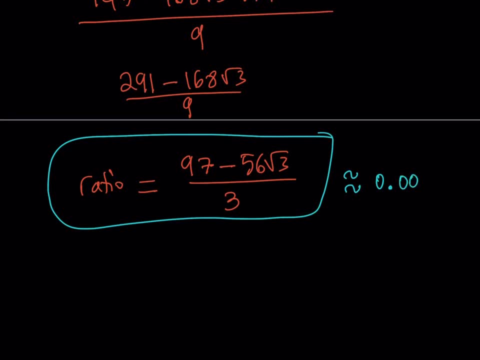 like. it's approximately 0.0017.. All right, Awesome, Great. Thank you so much for watching And I'd like to see your comments and I'll see you in the next video. Until then, take care, Bye-bye.